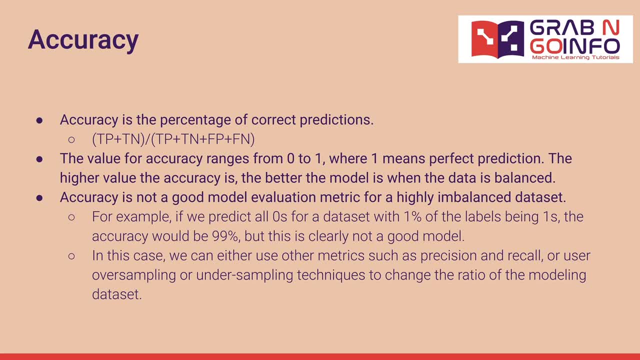 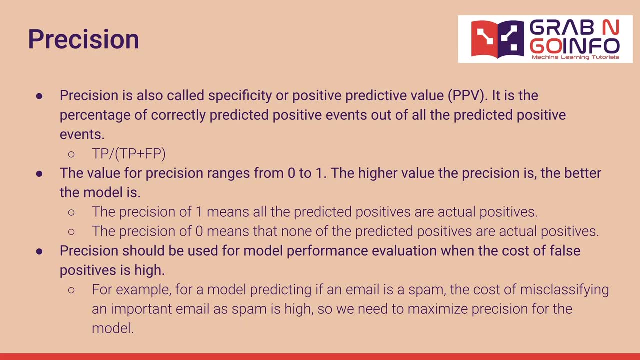 precision and recall, or user oversampling or undersampling techniques to change the ratio of the modeling dataset. To get the written version for this tutorial, please check out my blog post on mediumcom. I will put the link in the video description. Mediumcom is my most. 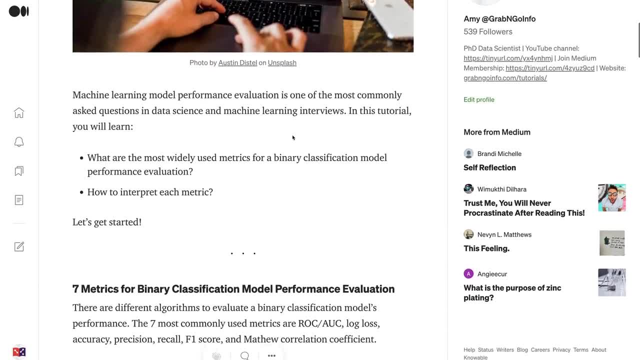 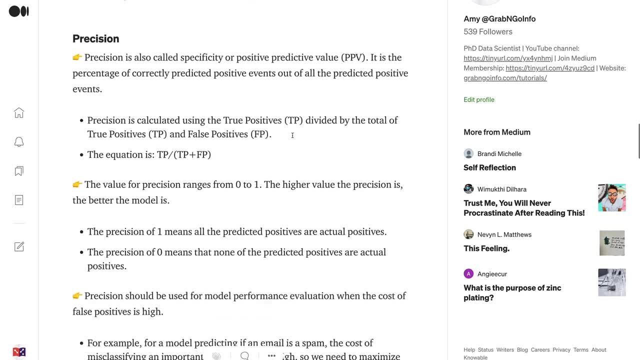 referenced website for data science and machine learning. It charges $5 per month for full access. I have been a mediumcom member for many years and that's the best $5 I spent every month. If you would like to learn more about mediumcom, please visit the link in the description. 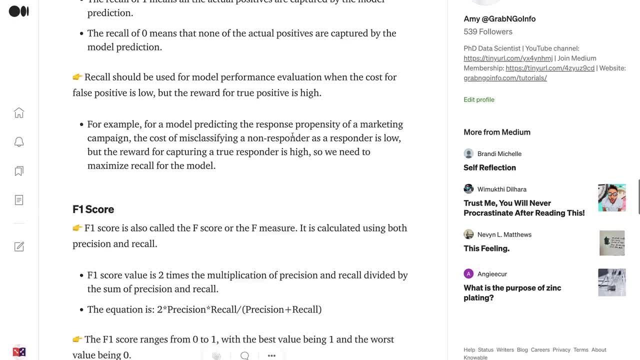 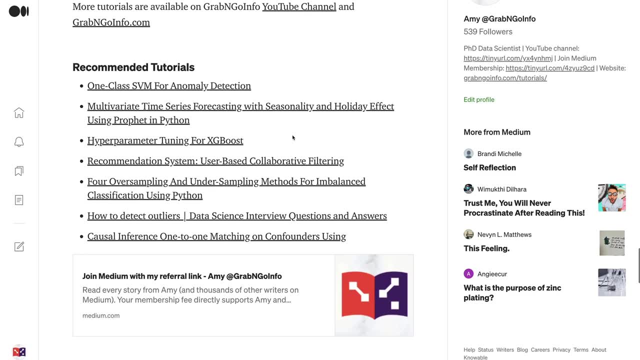 If you would like to support me as a content creator and buy me a cup of coffee, please use the link in the video description to join the medium membership at no additional cost. If you prefer not to join, you can still read the post, because there are a couple of free. 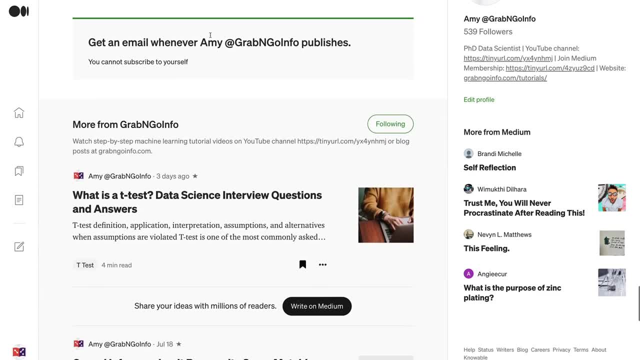 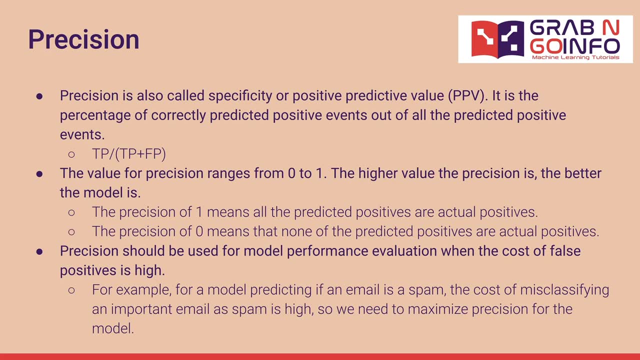 posts each month for everyone to read. Ok, let's continue. Precision is also called specificity or positive predictive value. It is the percentage of correctly predicted positive events out of all the predicted positive events. Precision is calculated using the true positives divided by the total of true positives and false positives. The 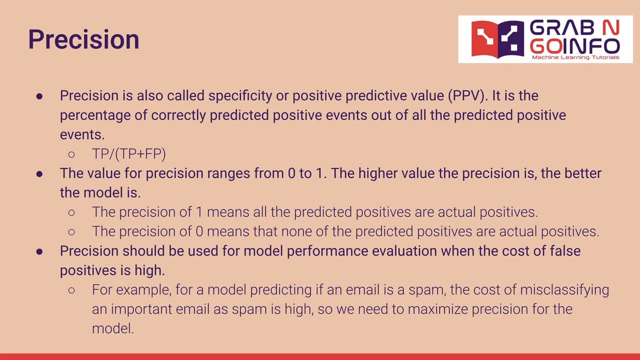 value for precision ranges from 0 to 1.. The higher value the precision is, the better the model is. The precision of 1 means all the predicted positives are actual positives. The precision of 0 means that none of the predicted positives are actual positives. Precision should be used. 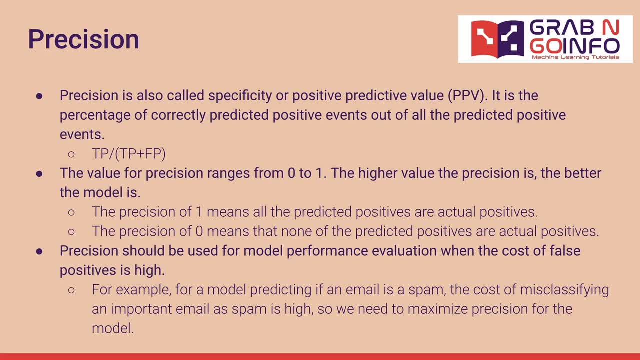 for model performance evaluation when the cost of false positives is high, For example, for a model predicting if an email is a spam. the cost of misclassifying an important email as spam is high, so we need to maximize precision for the model. Recall is also called sensitivity or true positive. 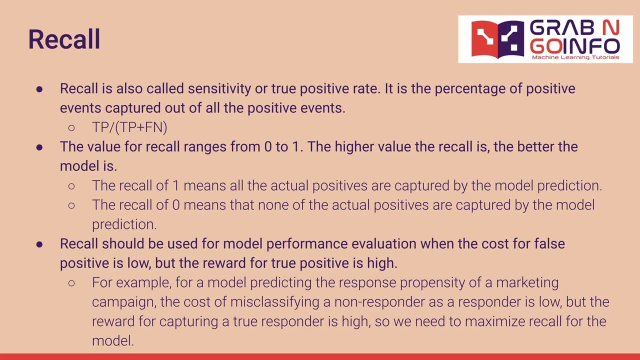 rate. It is the percentage of positive events captured out of all the positive events. Recall is calculated using the true positives divided by the total of true positives and false negatives. The value for recall ranges from 0 to 1.. The higher value the recall is, the better the model. 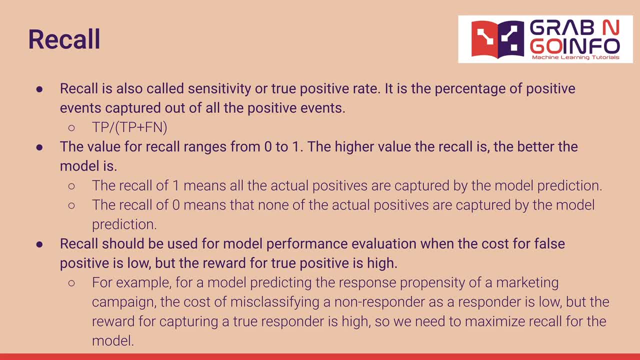 is: The recall of 1 means all the actual positives are captured by the model prediction. The recall of 0 means that none of the actual positives are captured by the model prediction. Recall should be used for model performance evaluation when the cost for false positive is low but the reward for true.